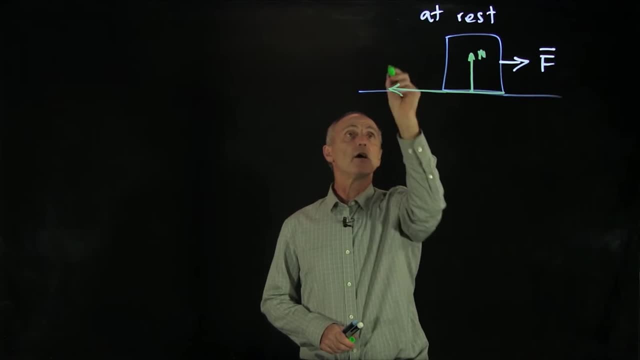 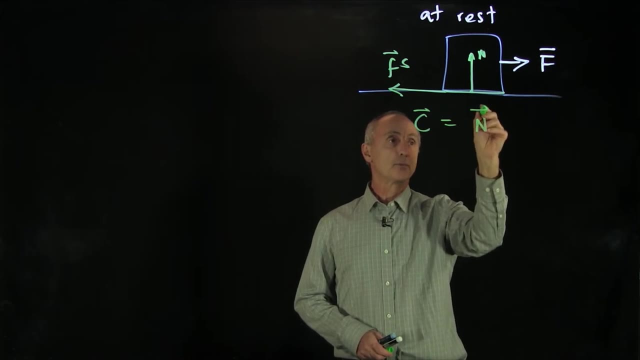 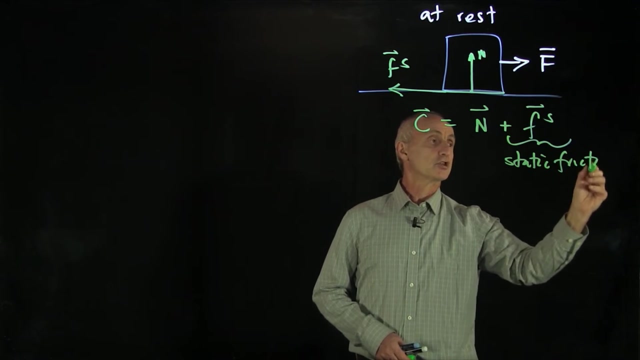 rest. the contact force now is what we call static friction, the tangential part of that, and the contact force is still the perpendicular part, the normal force plus the tangential part which we refer to as static friction. Now what happens with static friction is: 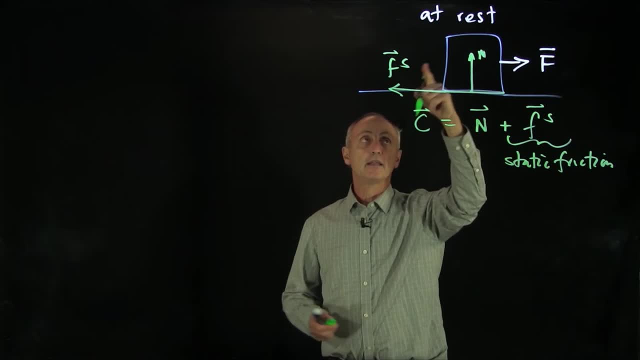 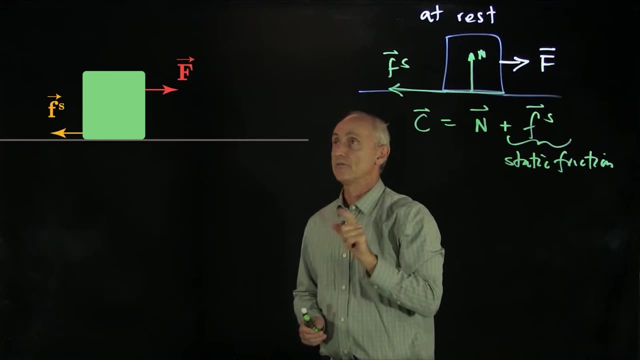 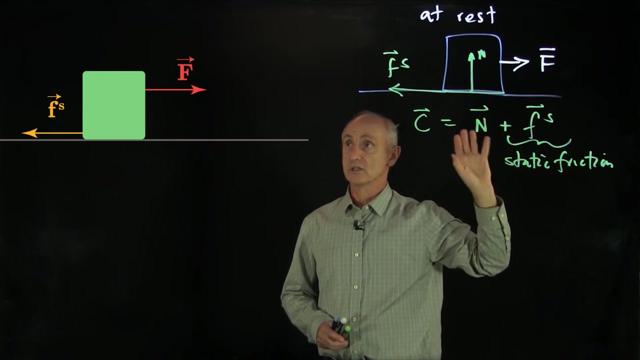 that if we don't apply a force at all, then there's no static friction. In fact you can see in this simulation That if we slowly increase the applied force, then the static friction force gets bigger and bigger. It depends on what we're doing to the system, But at a certain point, when 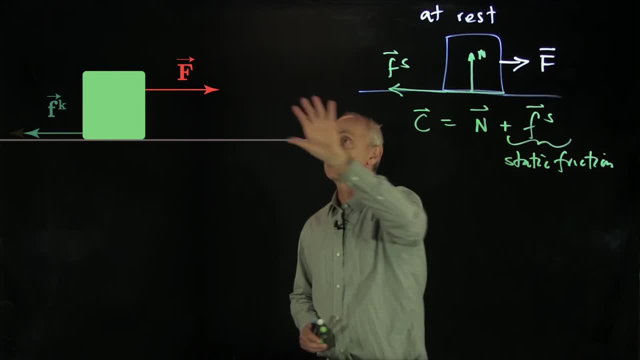 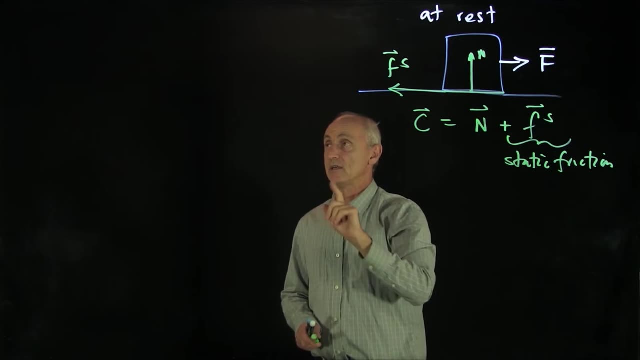 we apply a large enough external force, the object suddenly starts to slip. That's what we call the just slipping condition, And the reason for that is static friction has reached its maximum possible value. That has to do with the physics of the interaction between. 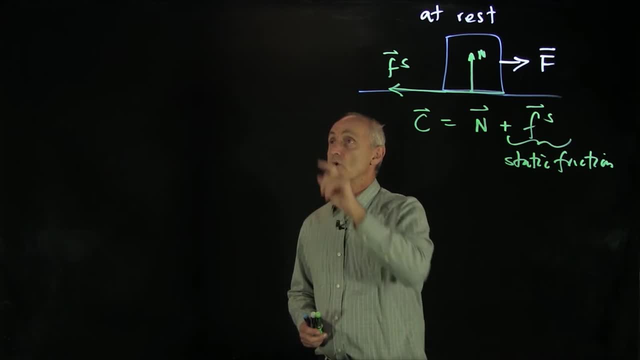 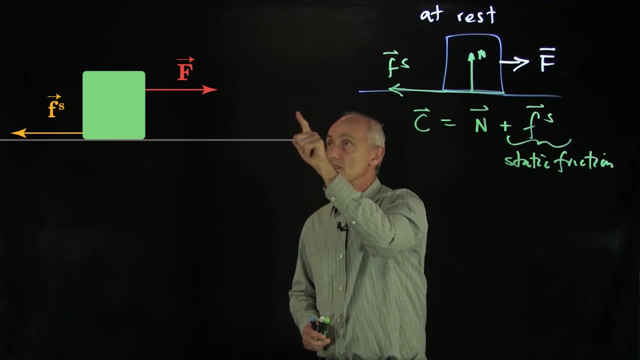 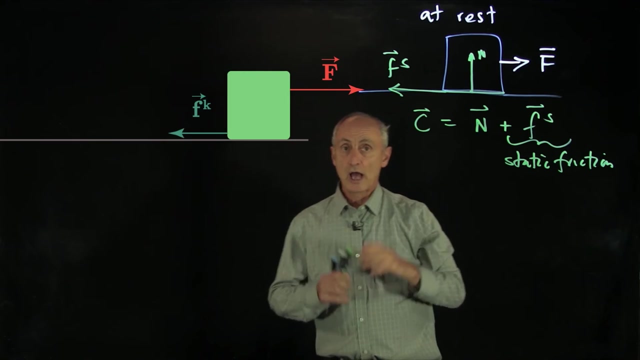 the surface and the object. So also there's a very subtle thing. is that, as you see, when we pull the force and it just slips, suddenly the friction has gone from static to kinetic friction and it's gotten a little bit smaller. How do we express those properties? Well, 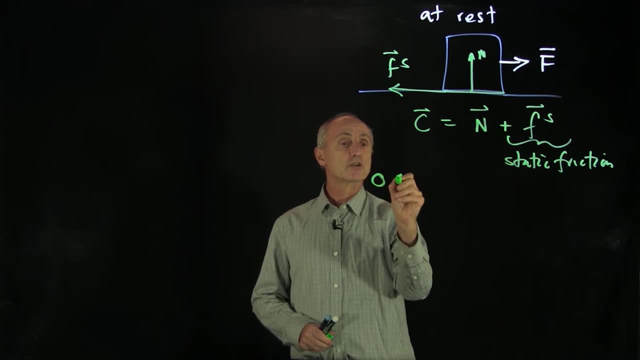 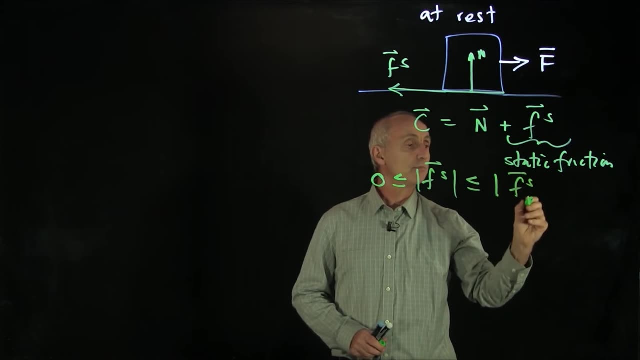 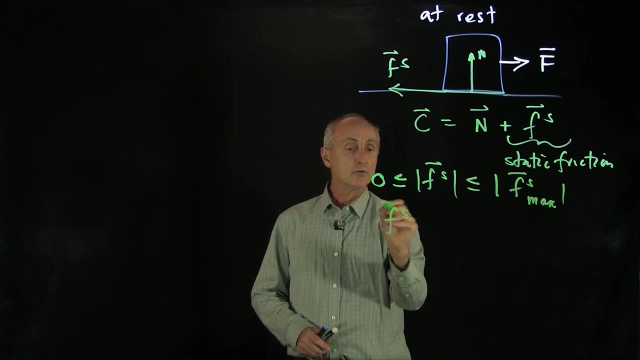 what we have is the idea that the static friction can vary in magnitude between zero and some zero, And that's because the momentum of static friction is less than or equal to the force that's got to be applied. And so now we're thinking about the force that's. 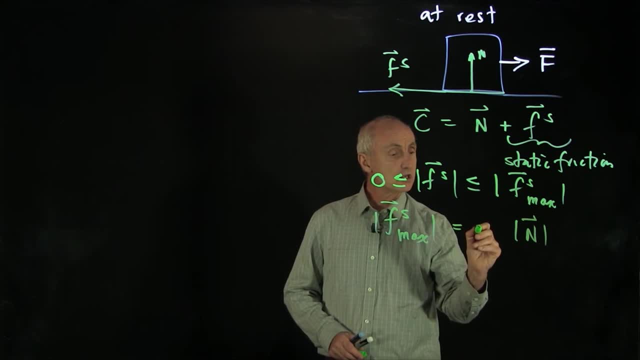 going to be applied. So we're talking about a force law And the force law in the law of law, and this is the Kierkegaard's Law of Magnetic Length, and this is the Kierkegaard's Law of Magnetic Length, and this is the Kierkegaard's law of Magnetic Length, and the force is equal. 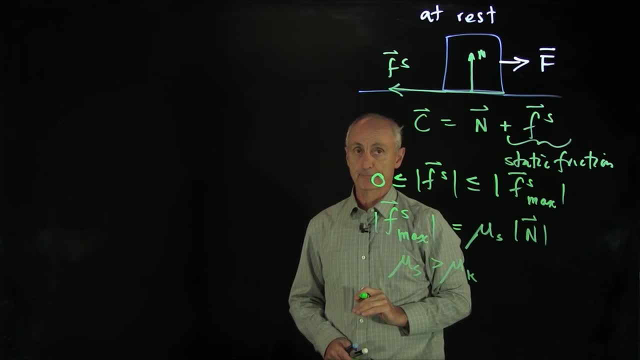 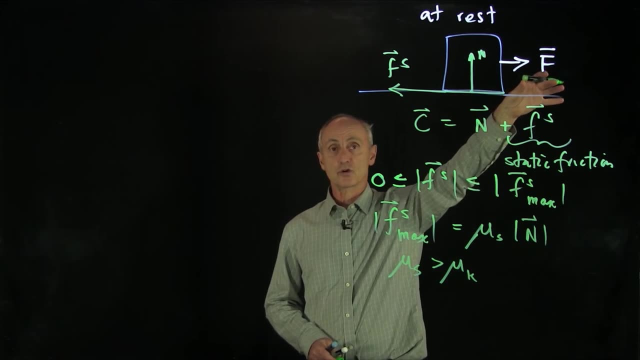 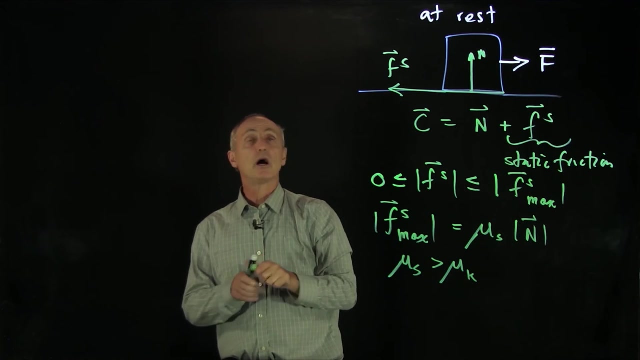 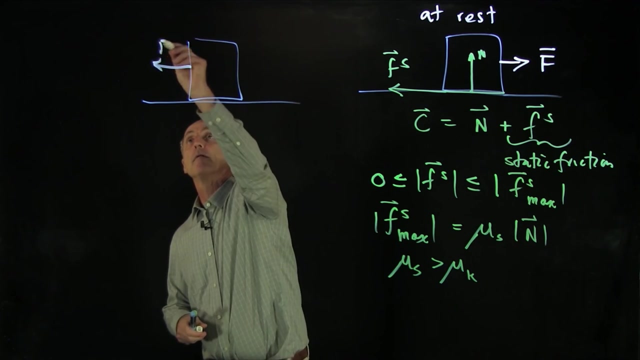 to the force got a little bit smaller when it just started to slip. Now, again, like kinetic friction, static friction is opposing this external force And, depending on the direction that the object moves, for instance, if we applied the external force in the opposite direction here, then